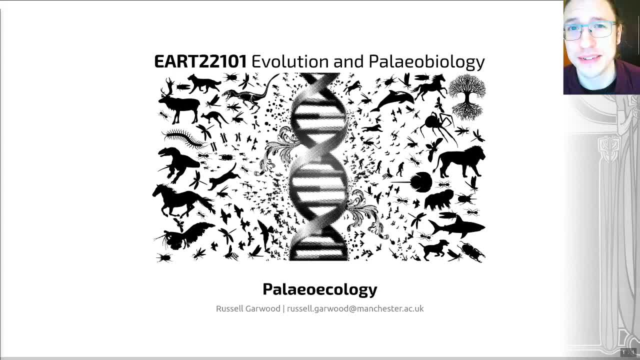 off by saying: why does this all matter? Well, let me tell you why this matters. Wasn't that a smooth seek? So I think this is actually really important because we can use ecology to explain both the distribution of living taxa across the globe, but also the distribution 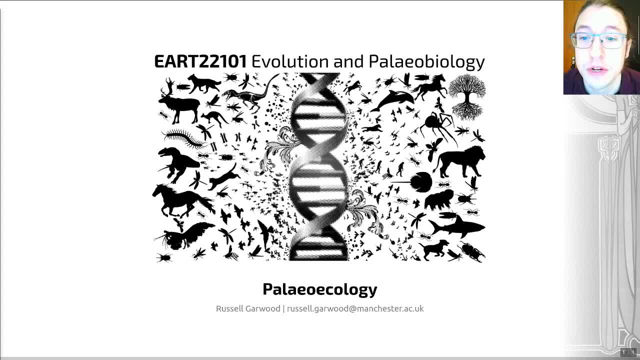 of fossil taxa across the globe. This tells us, for example, what environment rocks were deposited in, but it also looks at how those spatial relationships have changed with time and the factors that have influenced different animal communities and ecological communities- not just animals in deep time. 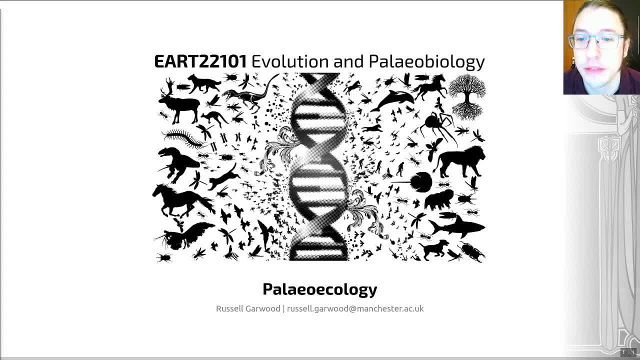 in the geological past. We don't get that without looking at the fossil record. Paleoecology is thus key to understanding ecosystems in the past and the life systems that were around at that time, But that in and of itself is only part of what paleoecology can give us By taking a 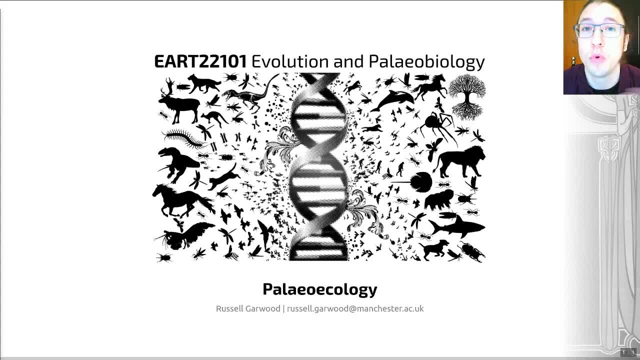 nuanced approach to this and looking at these questions broadly. we can also look at past climates, how they have changed, but then also how the biosphere, the things that are living at any given time, have responded to those changes in climate and in earth conditions. 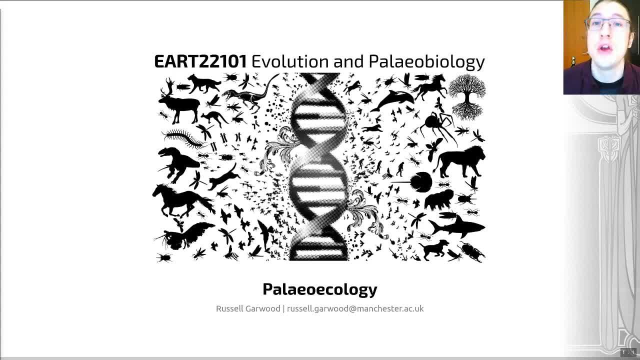 And in a time period, the modern day, where we are causing a series of changes to the environment of our planet, looking to the fossil record to understand how the climate is changing and how animals, organisms more generally, respond to changes in climate is a key thing that paleoecology can provide us with. 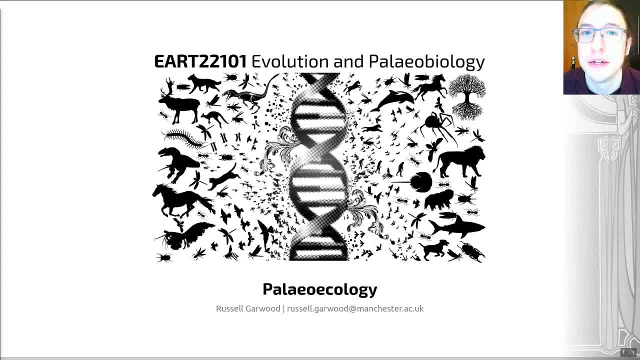 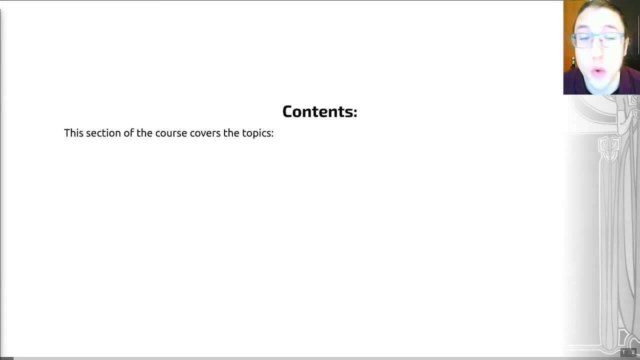 Some key information to help us understand the impact that we are having on ecosystems today and the likely response of those ecosystems to that forcing. For that reason, I think this is a really exciting and important topic and I hope you will find it interesting To provide you with a quick rundown of what we are going to be looking at over the series. 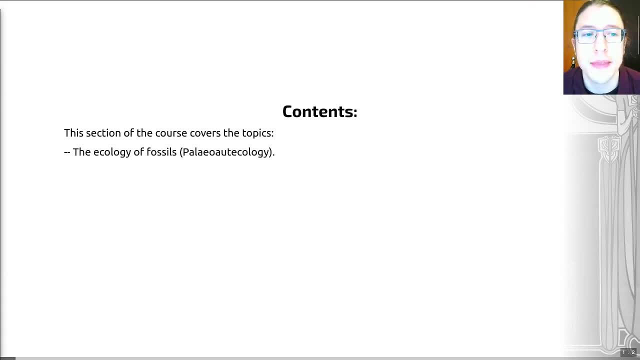 of the next few videos. we're first going to be looking at the ecology of fossils. so this is a thing called paleo autoecology, and by by that what i mean is actually understanding the ecology of individual species. if we look at a fossil and we understand its morphology, that can tell us.